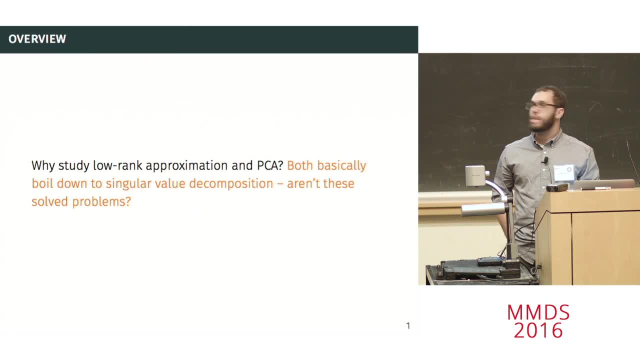 analysis. They're used all over the place, But in the vanilla setting they're both basically solved by doing a singular value decomposition, And this is something that has been studied in the numerical and your algebra community for decades. There's lots of really well-developed 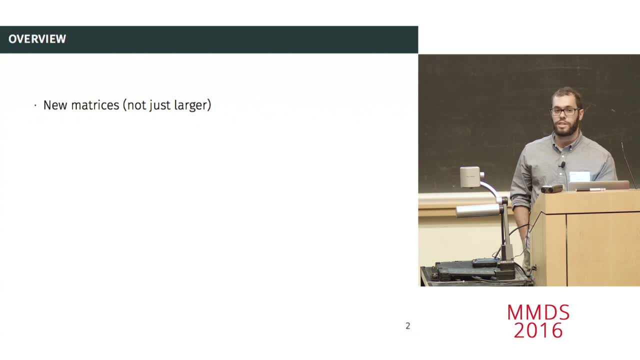 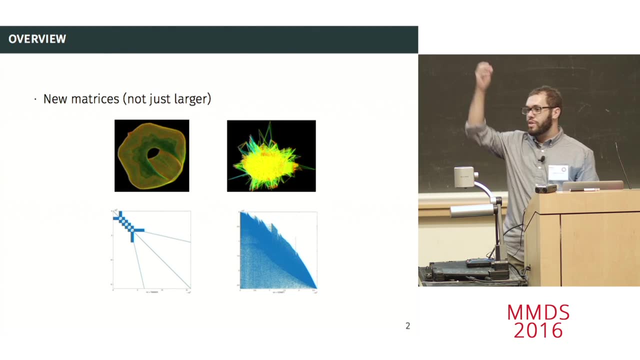 implementations. There's lots of really well-developed theory, So why am I still studying this problem? Why do I still think it's interesting? There's a couple reasons for this. Number one is sort of the obvious, just that we're working on different types of data sets. Not only are 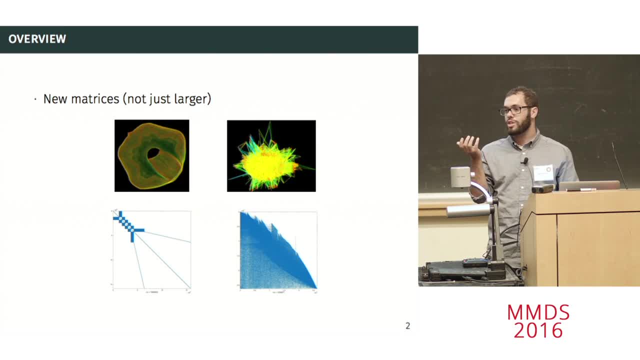 they larger. they're not always larger, but they also, For example, are much less structured. So there's tons of work on speeding up SVD algorithms for structured matrices And obviously there's a lot of SVD algorithms that don't take into 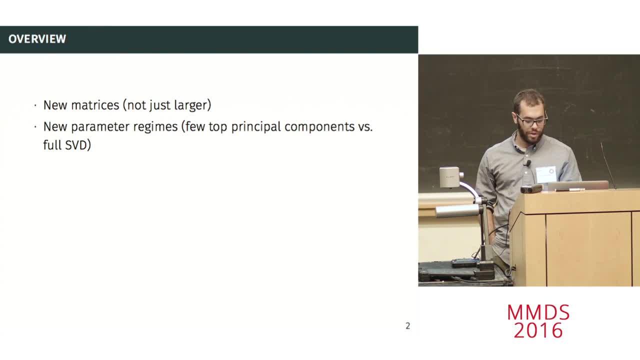 account structure, but there's maybe less work that could be done for dealing with unstructured matrices. There's sort of new parameter regimes. You're computing different numbers of singular vectors And one of the most important parameters is error. So error parameters are also changing. 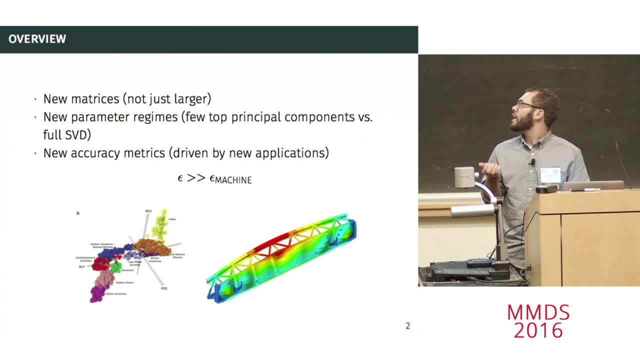 There's new accuracy measurements for new applications, And there's sort of two reasons. there's new accuracy metrics. Basically, there's this intuition that in machine learning and in data analysis generally, you set your error, your epsilon, to be much greater than 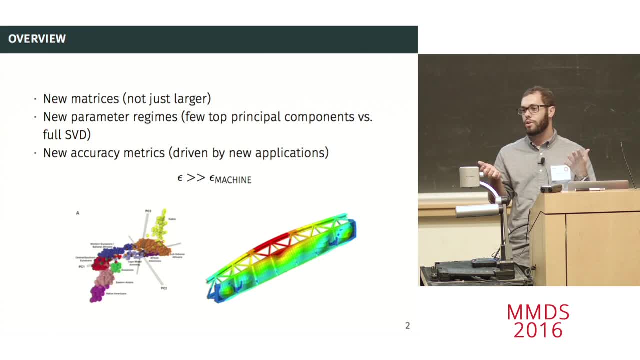 machine precision. So you're willing to tolerate basically larger error tolerances, and then you can look at different types of algorithms that give you these sorts of error tolerances. But it's not just that you're willing to tolerate larger error, There's just different ways. 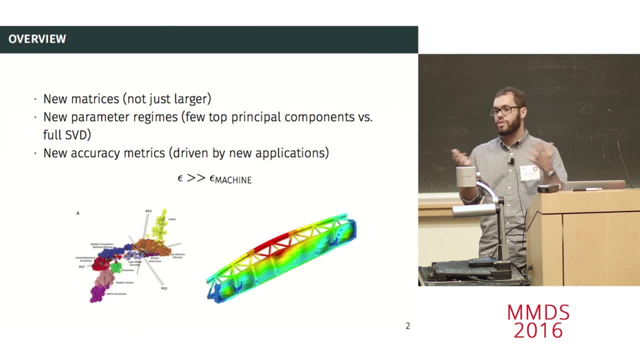 of measuring error. So if you're computing an eigenvector for some sort of scientific simulation, that eigenvector might have a physical meaning and you want to somehow approximate that eigenvector. If you're computing an eigenvector because you're using it as 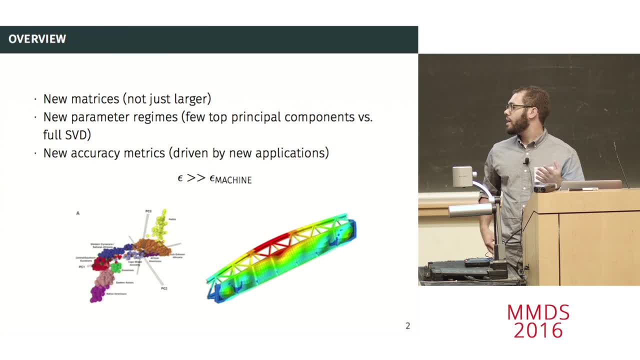 a principal component. there's no real physical meaning. It's sort of like it's a tool for visualization or classification or something like that, And so you should be measuring what is a good principal component using a different type of error metric than is traditionally. 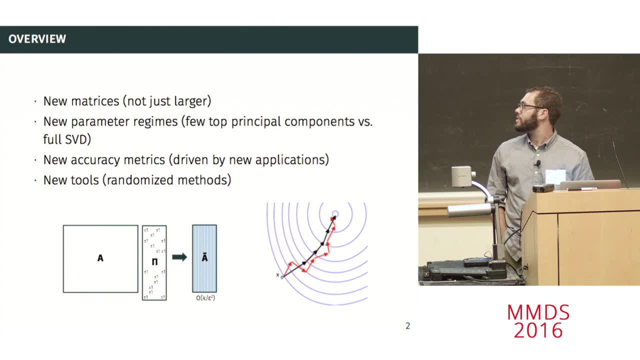 studied. It's not just that epsilon is bigger, Like epsilon should be different, basically. And then the final thing is new tools. So the thing that I look at most probably is randomized methods. So the biggest thing, that something that I work on a lot and some people 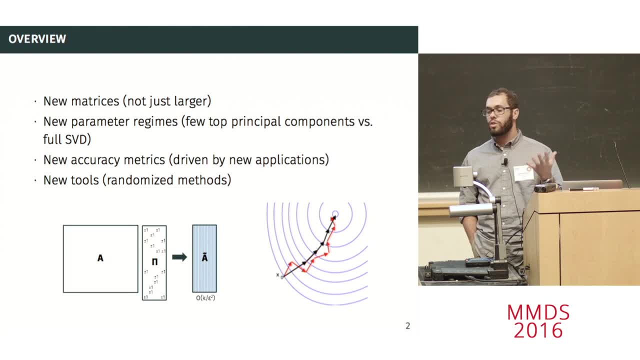 here work on. a lot is basically randomized sketching, which is basically: I have a large data set. I want to do a low-rank approximation or a principal component analysis of this data set. I choose some random matrix, independent of my data set. I multiply it by my data set. 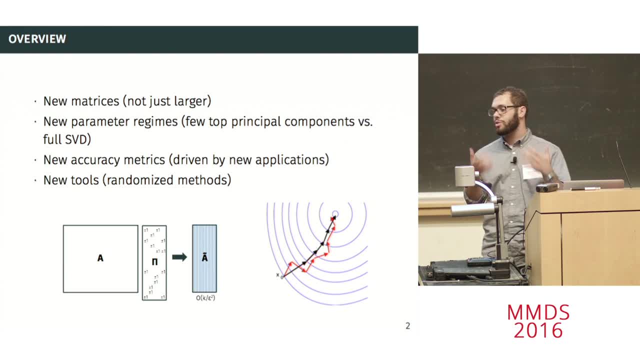 and I get this sort of randomized compression And from this compression I can still extract enough information to do some sort of reasonable data analysis. So this is one really widely used randomized tool that I'll talk about in a bit, And then another randomized tool which is not really new, but there's been a lot of interest and a lot of results. 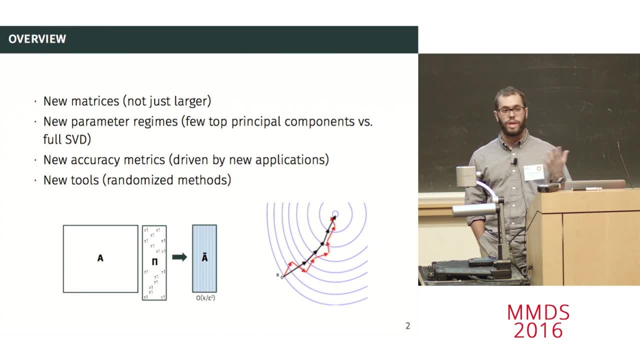 recently are basically on stochastic optimization methods and stochastic gradient descent methods. So these are basically: you're doing optimization via gradient descent, but you're saving time by not computing full gradients at each step. And there's lots of really interesting bounds here. They actually can give like, for example, if you're solving linear systems using these. 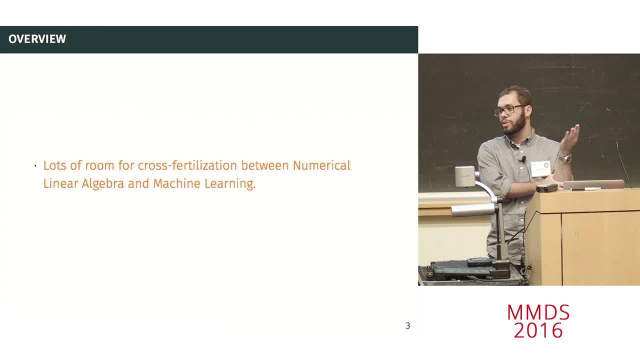 methods you can get just different bounds than you would get with traditional, like polynomial-based solvers. So I think there's tons of work to be done here. So these are two methods I'll talk about in a bit. Okay, The main point of this talk, which I hope I'll get across, is that I think that even 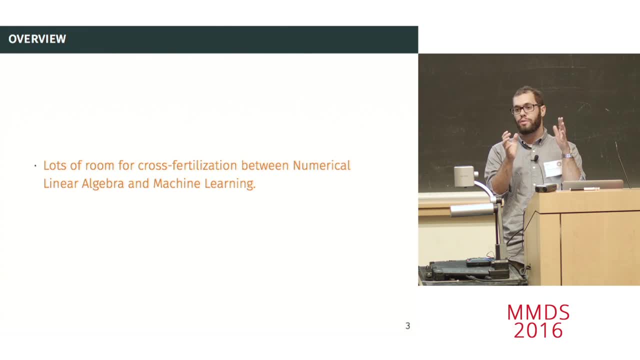 though lower-rank approximation and PCA are super well-studied, there's still a lot of room for cross-fertilization between what's known in numerical linear algebra and what people are doing in machine learning and data analysis, And I'm going to basically try to. 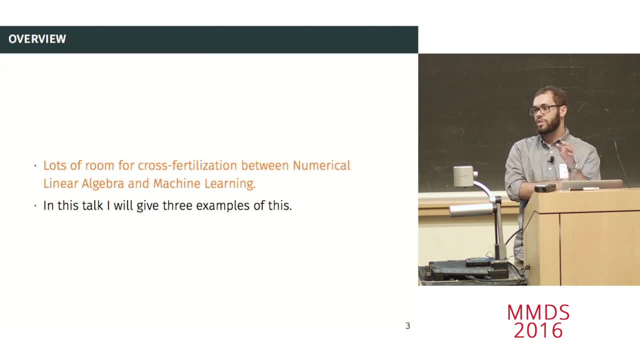 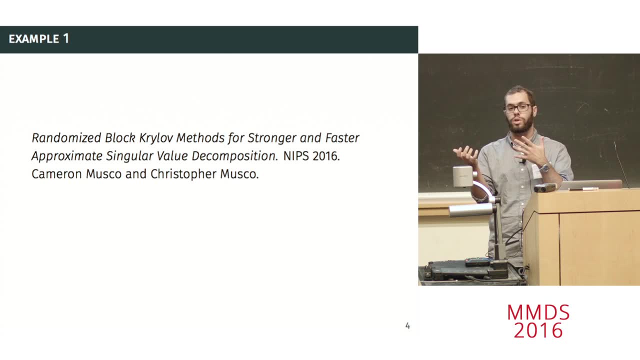 give like a couple examples of this in the talk. I think basically not everything has been solved on these problems but at the same time there's a lot of stuff that's been done in numerical linear algebra that can be ported over to data analysis and machine. 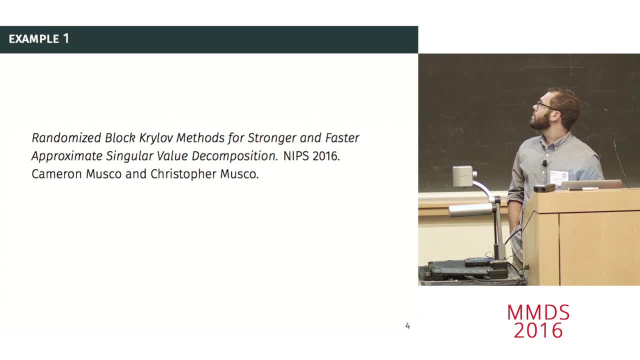 learning and give a lot of new understanding. So let me give you some examples. Okay, How many of these numbers were supported in the first study? It's a lot, Yeah, a lot. Could you give me a little bit of data this time? 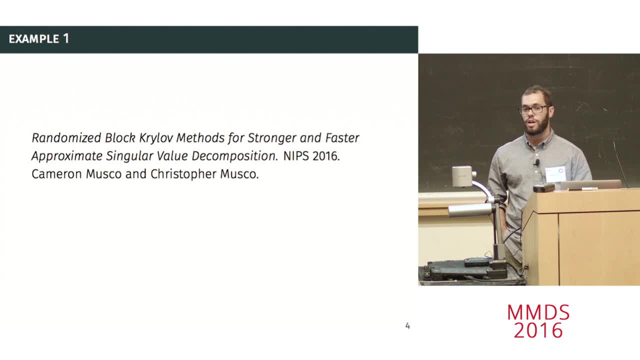 Sure, Okay. So first example: I'm going to talk about this paper from NIPSA last year with Chris Muzko on randomized block Krylov: methods for approximate singular value decomposition. So let me try to give you background on the singular value decomposition. Probably a lot. 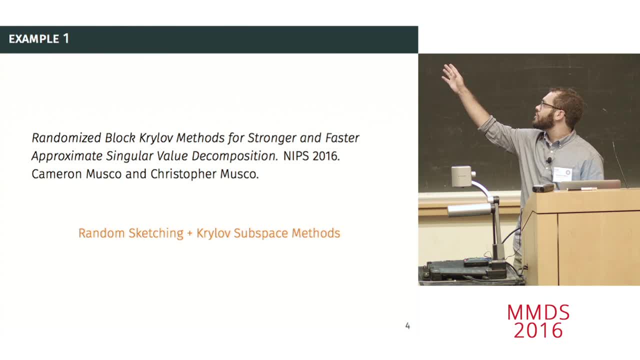 of people have seen it, but I don't know if everybody has seen it. Oh wait, Actually sorry. So what this is going to combine, if you forget everything I said about this. I'm trying to combine randomized sketching methods which have been really big in the theoretical computer. 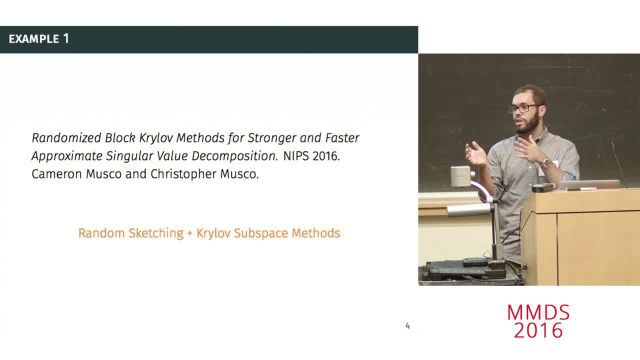 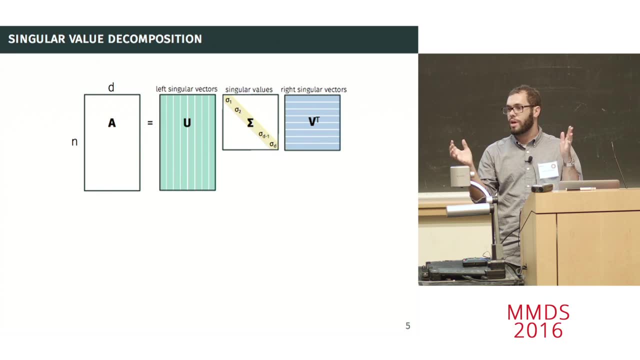 science area And I'm trying to combine these with basically traditional Krylov subspace methods and showing that by combining these methods we can get better bounds for low rank approximation. That's the high level of what this paper is trying to do. 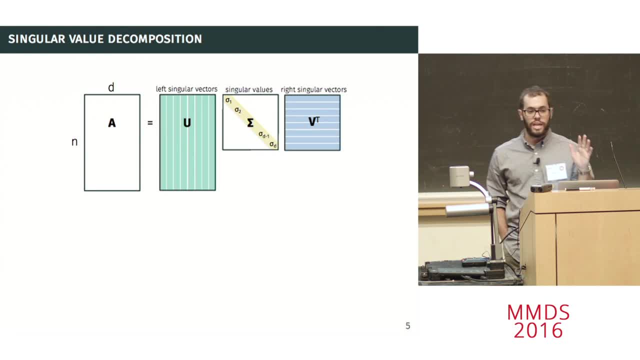 So what is the SVD? It's something I can apply to any matrix. I take any matrix A and I can decompose it into the product of three matrices. Basically, U has orthonormal columns, which are the left singular vectors of the matrix. 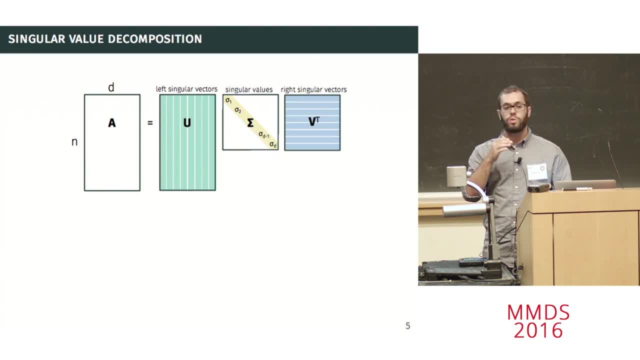 They span It's column. span V has orthonormal rows. They're the right singular vectors of the matrix. And then sigma is a diagonal matrix, It's non-negative And it contains the singular values of the matrix, usually basically ordered from sigma 1, which is the largest. 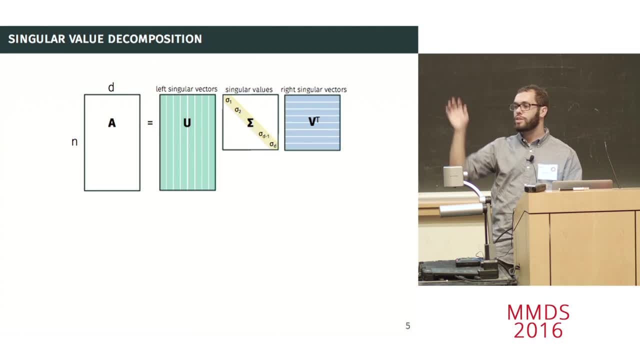 to sigma d. Now, this is principal component analysis. The singular vectors are the principal components of the matrix, And so this is why this is very useful. Those principal components corresponding to larger singular values are the important principal components. They're sort of the directions of largest variants. 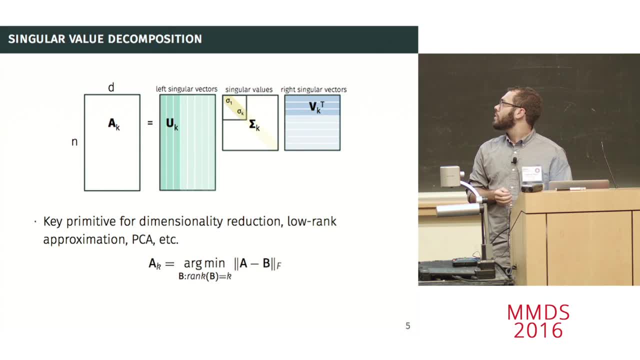 within your data set. Also you can directly read, You can read off optimal low-rank approximations from the SVD. So if I just take my matrix and I basically zero out all but the top k principal directions, I get this rank k matrix Ak which. 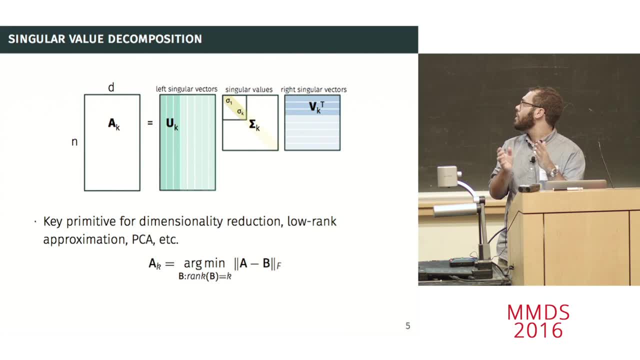 is the best k-rank approximation of my matrix in many senses. One sense is that if I look over all rank k matrices B, it minimizes the Frobenius norm distance between A and the rank k matrix B. So it's optimal in the Frobenius norm. 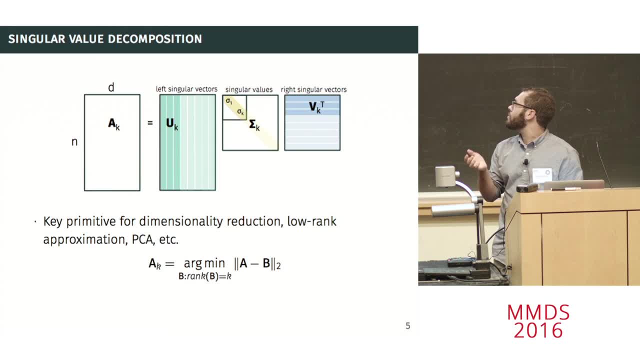 reconstruction sense of doing low-rank approximation. Another norm that is optimal And this is the operator norm. So this is an important norm for lower-rank approximation. So if I compute an SVD, not only is it giving me the top principal components of the matrix, 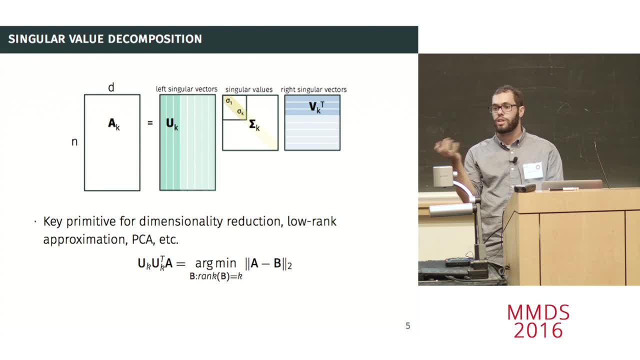 I can just read off an optimal lower-rank approximation And then I can plug in this lower-rank approximation to whatever application I'm using it in. Oh, let me just mention that the zeroing out of singular vectors is not always the way that people talk about this. 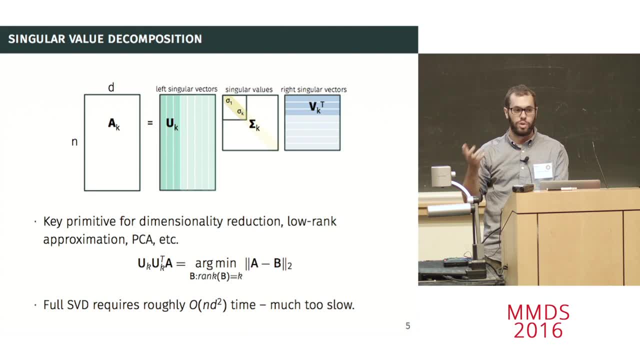 It's also equivalent to projecting onto the span of my top k principal components. Doing a full SVD, though, requires nd squared, So it's just totally. you can't do a full SVD for a large data set. It's like solving a linear system. 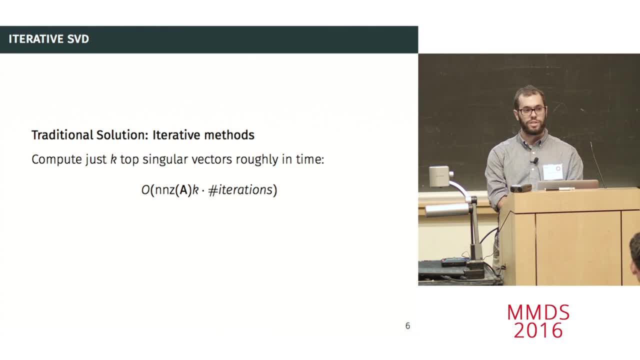 with Gaussian elimination. So you have to do something different, basically, And the traditional solution is iterative methods. So traditionally, if you're doing SVDs on large matrices, you're using some sort of iterative method. You're just going to compute k singular vectors. 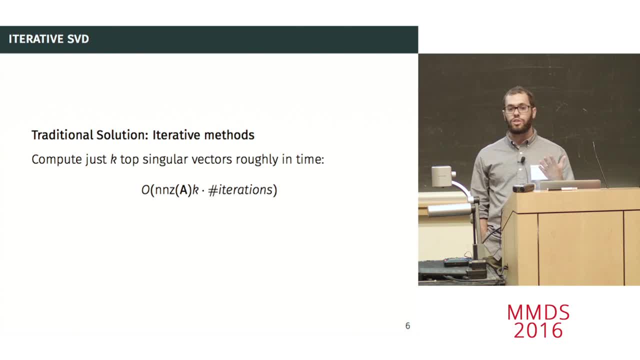 of your matrix or k principal components instead of a full SVD, And that's all you need for lower-rank approximation or PCA. The runtime is typically like the cost of an iteration which there's lots of different iterative methods, so I'm just being rough. 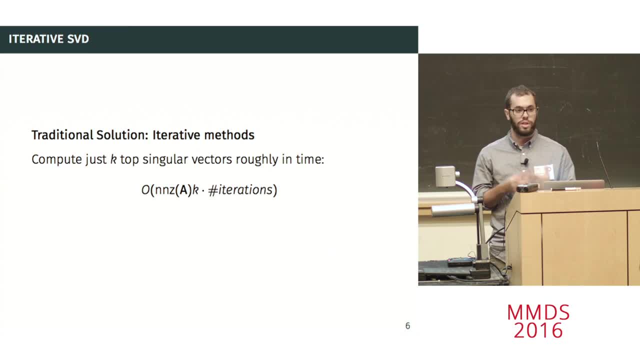 is something like doing k matrix vector multiplies So n and z a the number of non-zeros in your matrix times k, And then, whatever your iteration count which will depend on your error and your convergence rate and all sorts of things. 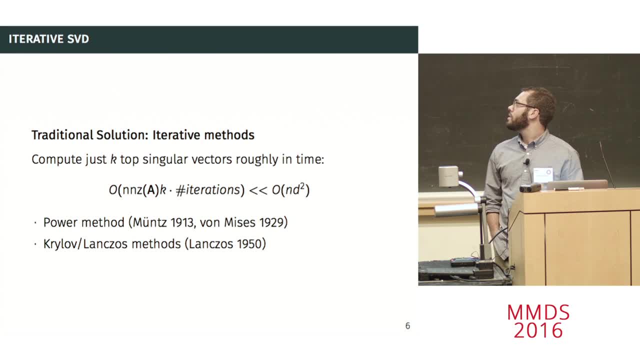 But typically this is much smaller than the cost of a full SVD, And the two iterative methods that most things are based off are basically a power method. So probably a lot of people have seen power method for, for example, computing the top eigenvector of a matrix. 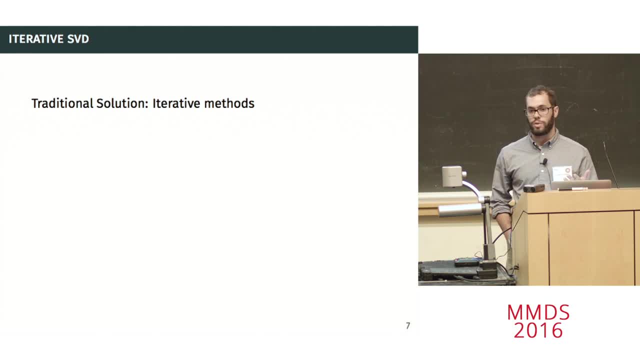 And then the Krilov and Lanchos methods, which are basically accelerated polynomial methods and sort of actually like the focus of what this work will be focused on. OK, So what sort of guarantees do these iterative techniques give you? First of all, you're looking for some top singular vectors. 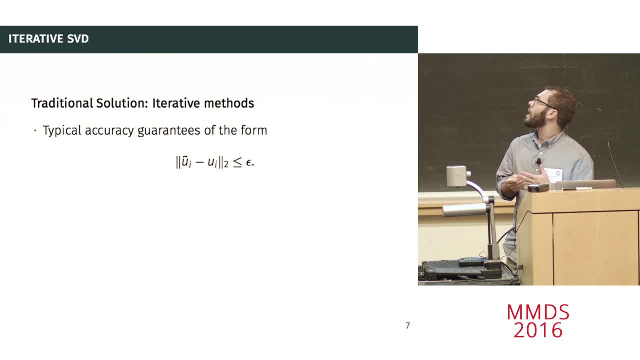 of your matrix And the sort of guarantees that they're going to give you are basically, if I compute an approximate singular vector like u, tilde i, I want to basically prove that it's going to be close to my true singular vector, ui. 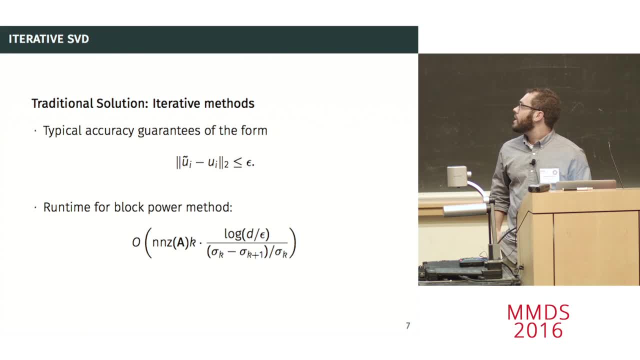 in some reasonable way. OK, So I'm going to call this integral norm like the two one, And the runtime ends up being something like the cost per iteration, which is this n and z a k term And the number of iterations, basically. 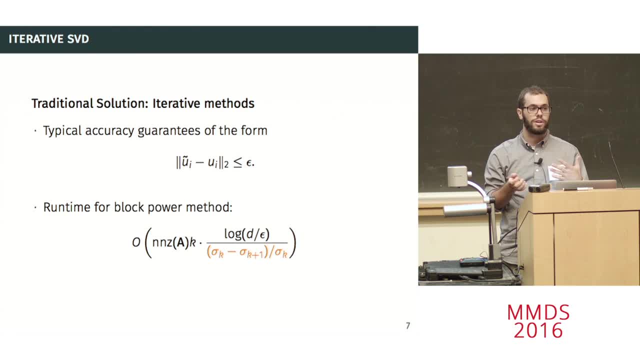 has this logarithmic term, which is because you're basically getting linear convergence on your error And then it also depends on your convergence rate And, critically, this convergence rate depends on the spectrum of your matrix. So it depends on whatever your input matrix is. 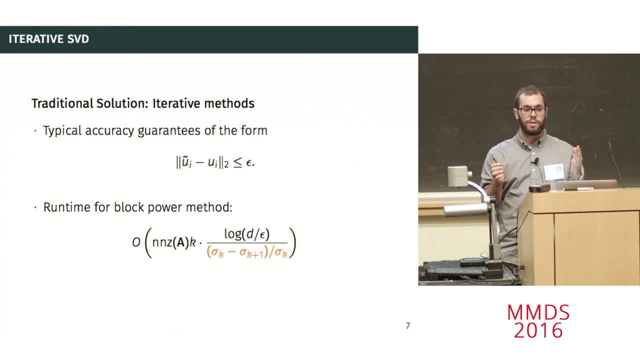 Specifically- this is an example just for power method, which is the most basic iterative method, But this sort of generally applies this sort of principle that you're going to depend on the spectrum of your matrix If you want to get convergence in that sort of error. 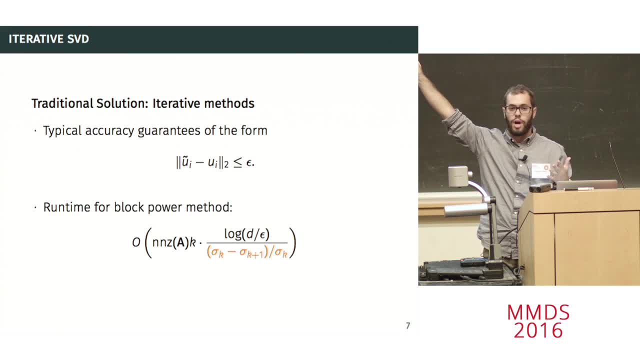 guarantee you're going to depend on what's called the spectral gap. So probably a lot of people have seen this with Markov chain mixing or just because you've looked at SVDs and eigenvector decompositions. It's basically the relative gap between your kth. 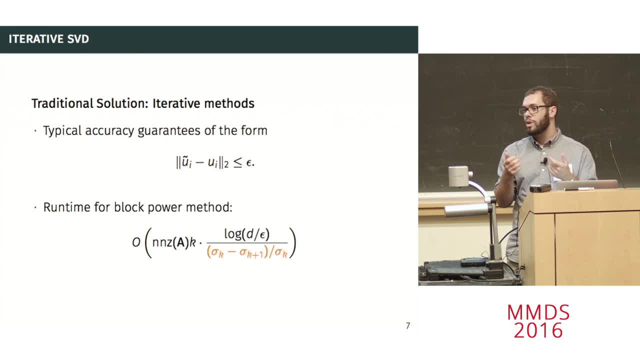 and your k plus first singular value. If this gap is small, those singular values are very close to each other And it's difficult for iterative methods to distinguish between the two singular directions. So basically, the smaller the gap is, the more costly the iterative method becomes. 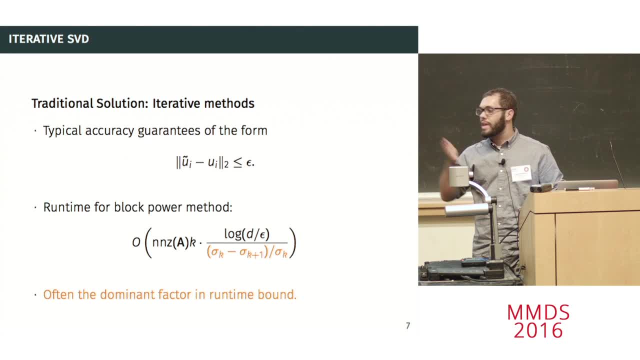 And it's sort of inherent. So sometimes it's just sort of included and thought of like a constant in a way, as it depends on the convergence rate. But it can often be the dominant factor in the runtime bound, Because often gaps actually are very small. 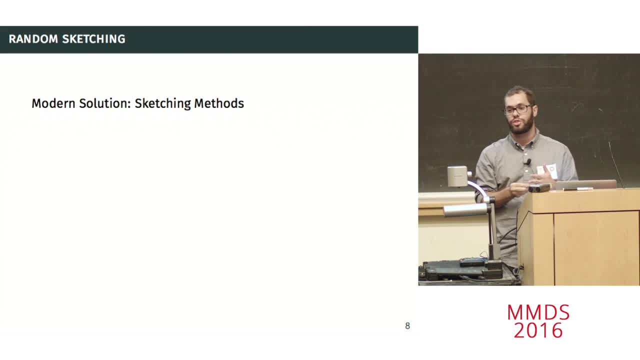 especially in data analysis applications, where you're not going all the way down to machine precision, So your epsilon is not necessarily all that small. So how do we remove this dependence on the spectrum of the matrix? So the modern solution which there's- 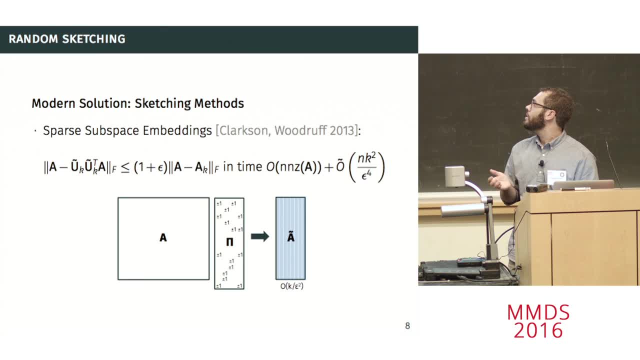 been tons of work on in the last maybe 15 years is randomized sketching, which I mentioned briefly. You have your original matrix A, You multiply it by a randomly chosen sketching matrix pi And you produce this sort of randomized compression of the matrix. 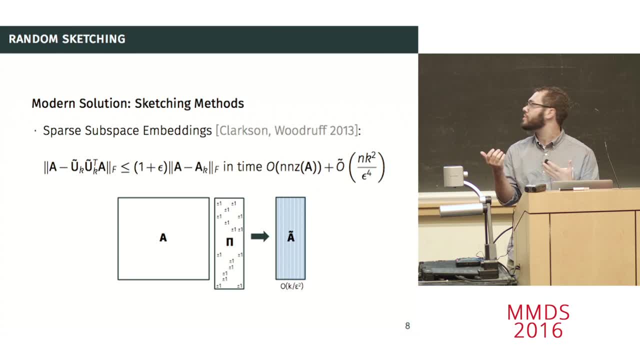 And depending on the distribution of pi, you can basically prove things about this sketch A tilde Specifically. you can prove you can extract good principal components from it. So one thing you can get is basically you get that you can get some principal components. u tilde k. 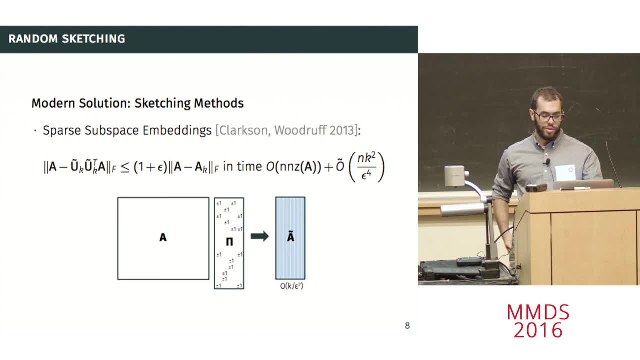 Such that if you project onto them, so A minus u tilde k, u tilde k transpose A. This is A minus its projection onto the principal components of essentially A tilde. So you essentially worked with a sketch instead of the original matrix. 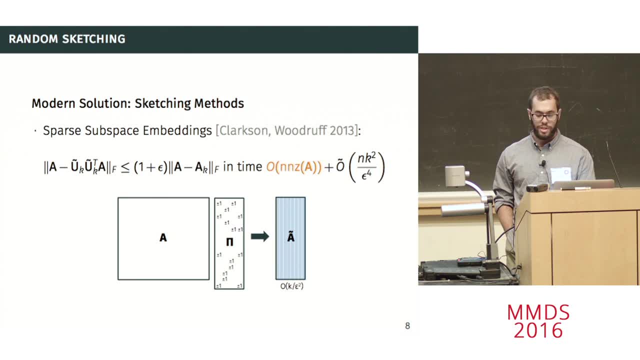 This Frobenius norm error is within 1 plus epsilon of the optimal for Frobenius norm error And you can get super fast runtime. So the dominant cost in the runtime is something like the number of non-zeros in your matrix. This is basically the time to multiply your matrix. 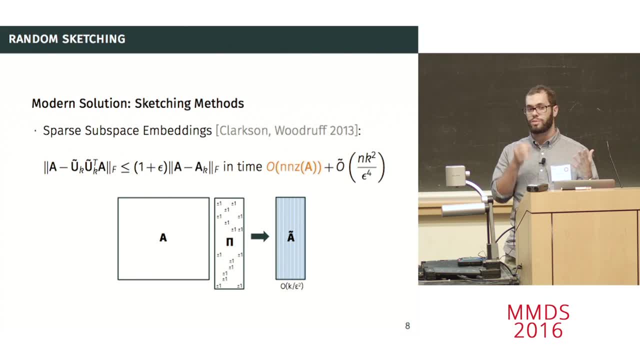 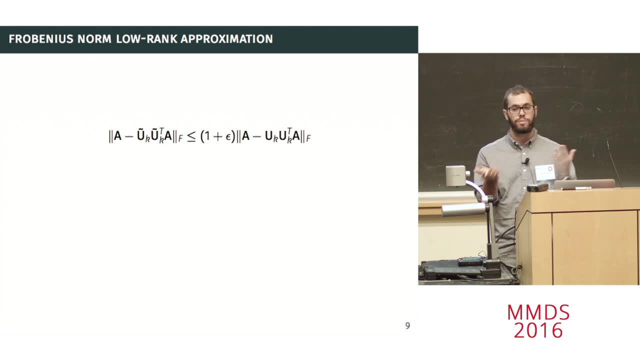 by this random sketching matrix. The sketching matrices are chosen so they're fast to multiply by, So specifically either structured or extremely sparse. So that's the dominant cost in your runtime, which is super fast. That's basically the time to read your matrix. 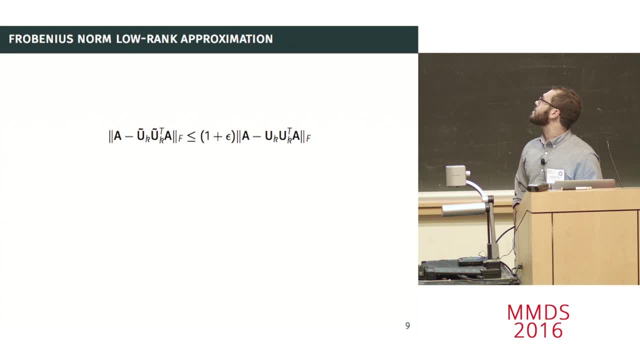 OK, But let's talk a minute about so you get really good runtime bounds. What is the deal with this Frobenius norm error guarantee? So this is one way of talking about a good lower anchor approximation. You've got a lower anchor approximation. 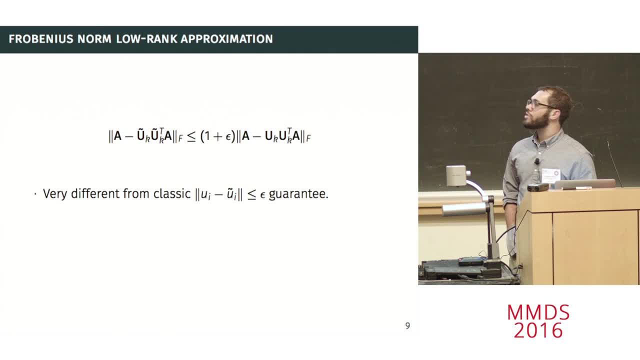 which is near optimal in the Frobenius norm metric. First of all, it's totally different than classical bounds on the SVD. So classical bounds on SVD algorithms are telling you: you actually computed good singular vectors, You don't need to have computed singular vectors. close. 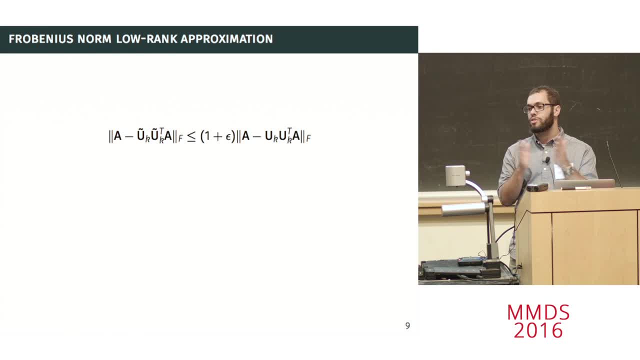 to the true ones to get a good lower anchor approximation. If there are two singular values that are close to each other, you don't really care about distinguishing them. You really just need to get one or the other. Second of all, it's sufficient in many circumstances. 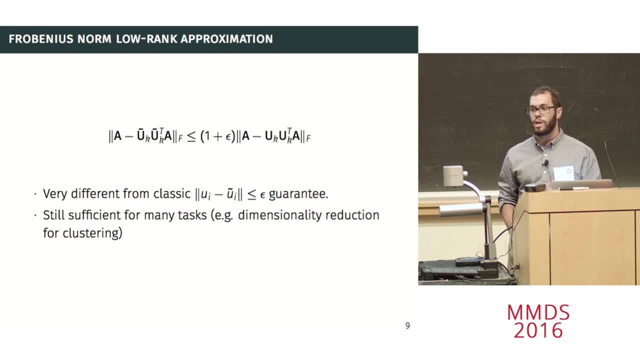 both. intuitively speaking, It's nice to get something close in the Frobenius norm. You can also prove sometimes it's sufficient for various clustering tasks, And so that's another thing. It's a really useful error metric and it's nice that we have really fast algorithms for it. 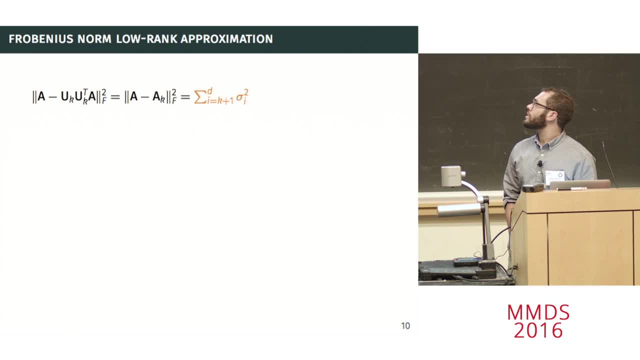 But it can be weak. The reason it can be weak is basically the Frobenius norm of a matrix. The Frobenius norm of a matrix is the sum of its squared entries. This happens to be equal to the sum of its squared singular values, or the sum 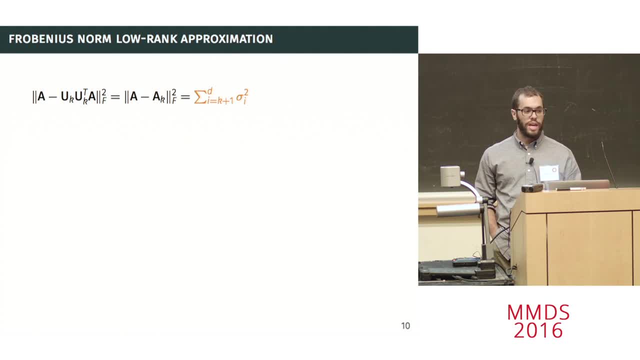 of its squared eigenvalues. If you look at the Frobenius norm of a minus its best-ranked k approximation, the best-ranked k approximation basically zeroes out the top k singular values of the matrix. So this Frobenius norm is the sum of the bottom eigenvalues of the matrix, all but the top k. 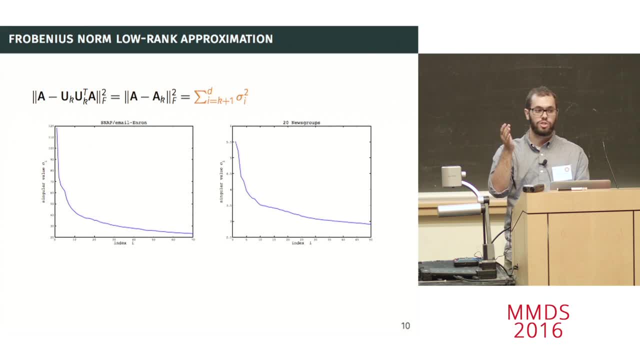 Most matrices display what you call spectral decay, which is basically that the larger singular values tend to be significantly larger than the smaller singular values. Almost all data sets have this, and this is why low-rank approximation is such a widely used tool, because, basically, the data set is in some sense. 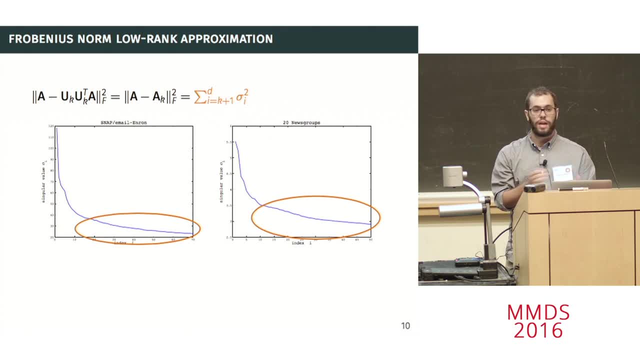 close to low-rank. But despite the fact that you have strong singular value decay, if you have a really high-dimensional data set and if your decay is not super high, super strong, this sum of small singular values can actually be very large. 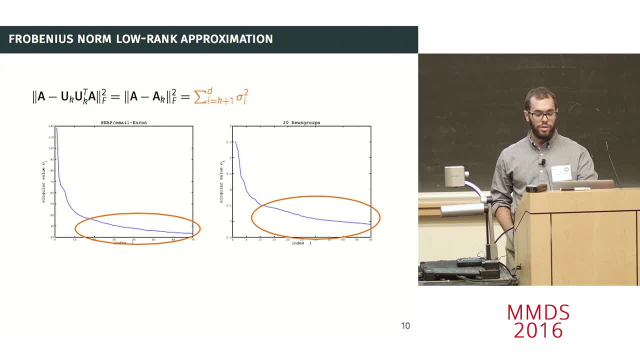 So basically, I call this a heavy tail of singular values. Even though there's a lot of decay and even though this is a matrix, you might care about doing a low-rank approximation for this Frobenius norm, error is very large. 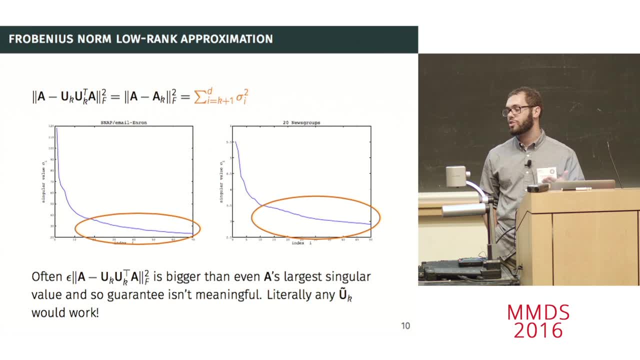 So it's another way of saying it- is that this matrix doesn't have a good Frobenius norm low-rank approximation. Often the size of the tail can be bigger than even the largest singular values of the matrix. so there are cases when the Frobenius norm guarantee doesn't. 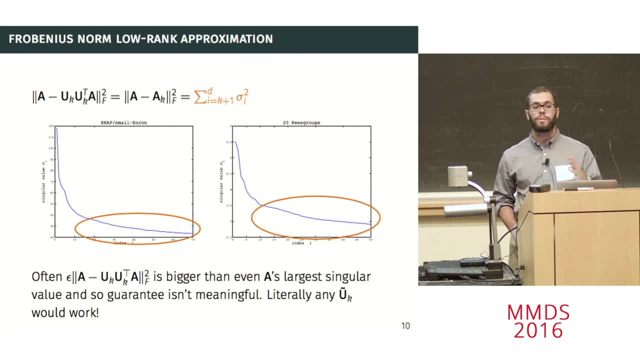 really give you any guarantee on the quality of the lower-rank approximation, even on matrices that you actually care about lower-rank approximating. So we want to solve this problem. That's what we set out to do is well, what if we want to still have a really fast runtime? 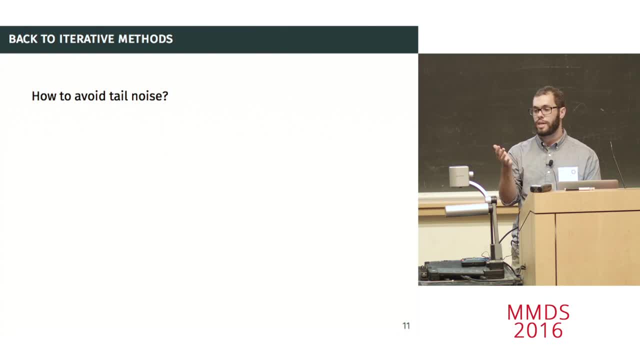 We don't want to depend on the spectrum of the matrix, but we want to do better than Frobenius norm in cases when it's weak. How can we avoid this? what I'm calling tail noise, this tail of smallish but still too large singular vectors. 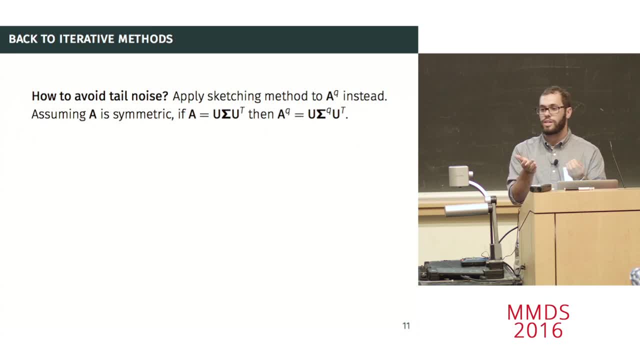 What we can do is instead of sketching a. so we are using linear, like these randomized sketching methods to get this error metric. instead of sketching a, we can sketch a raised to the q with power for some reasonably large q. 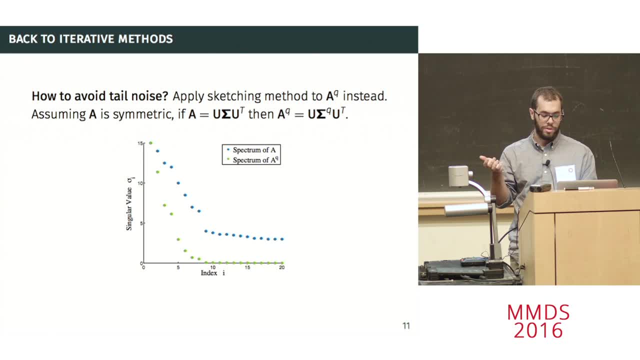 When you raise something to the q with power, it basically powers up its singular values. So if I plot the spectrum of a versus the spectrum of a raised to the q and I scale them so they have like the same top singular value. a to the q has a much stronger. 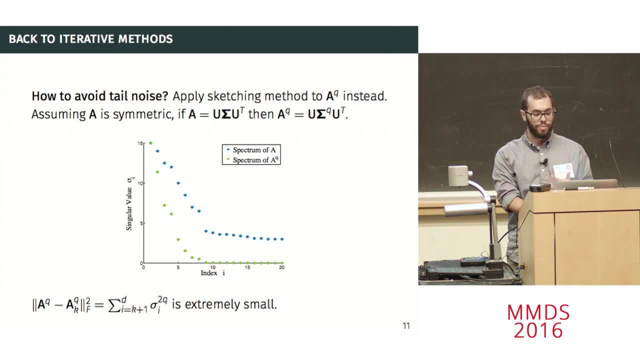 spectral decay because I've powered it up. So its tail of singular values is much smaller. Mathematically it means that the Frobenius norm error between a to the q and its best-rank k approximation is actually small compared to its larger singular values. 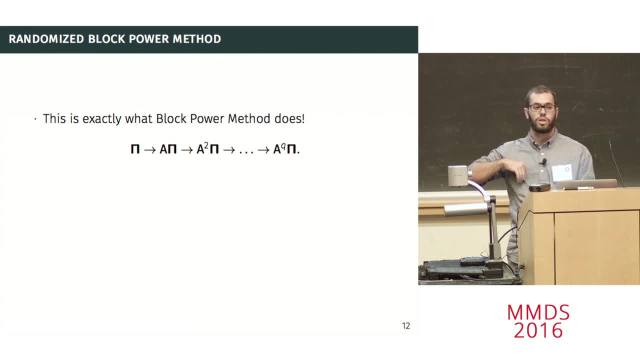 So if I perform sketching on a raised to the q with power, I'm going to get a good- basically good- singular vectors of my matrix. This is actually exactly what power method does. So it's not how people look at power method ever. 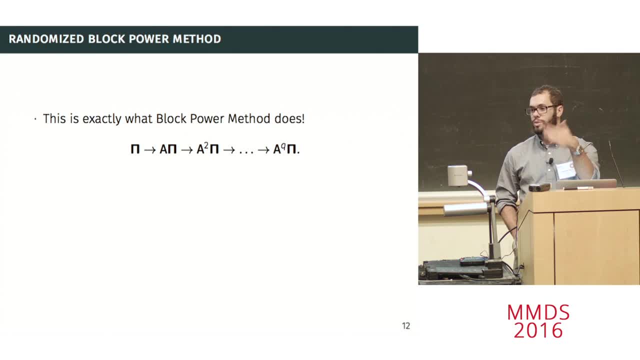 I mean so. usually you look at power method as you're applying your matrix to some vectors and this is causing your vectors to converge to the top singular vectors of your matrix. But another way you can look at it is: power method is just an. 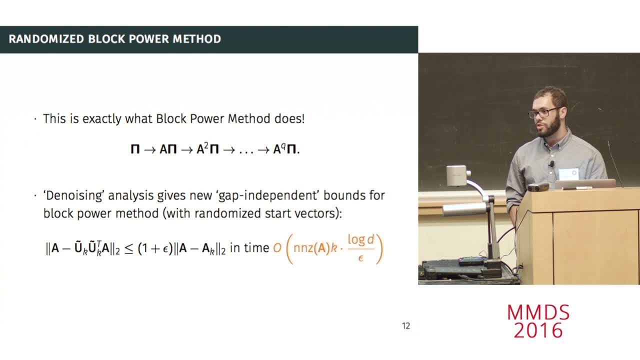 iterative way of applying a to the q times some randomized set of start vectors. This is like applying a very coarse sketching method to a to the q, And if you use this denoising analysis rather than traditional convergence analysis, you can basically show some interesting. 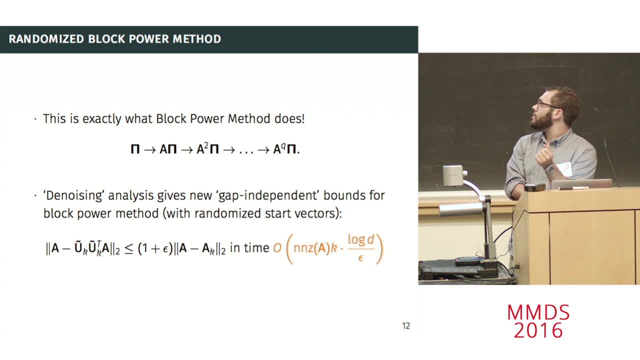 gap-independent guarantees for the power method. So basically, you can show that instead of getting near-optimal Frobenius norm error, you get this near-optimal spectral norm error for your lower-rank approximation, which is a much stronger notion of error generally speaking. 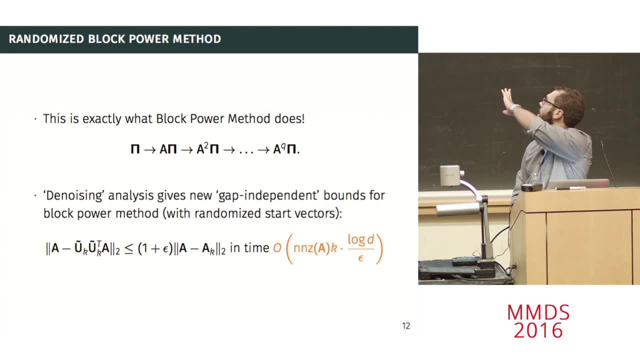 And your runtime is basically the iteration cost is nnz a, k and the convergence time is log d over epsilon, where epsilon is your error parameter. And this is basically. you run approximately one over. you set q to basically one over epsilon. 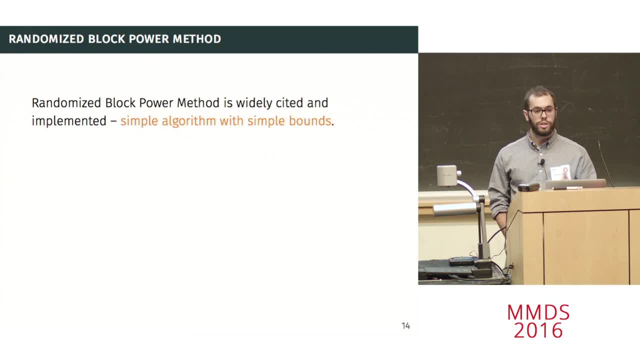 So there's no dependence on the matrix. it's just like a very simple runtime bound that gives you a very simple guarantee on your lower-rank approximation. There's been a lot of work on this and, importantly, I think it's really popular in the machine learning community. 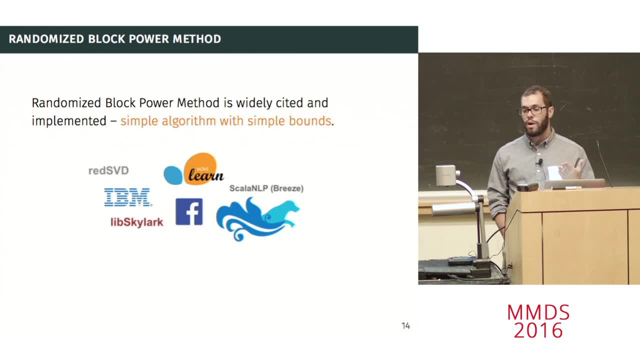 So there's tons of citations to these results on what's called randomized power method, which is basically power method, And it's implemented all over the place. Like a lot of people have started implementing it, It's because it's such a simple implementation. 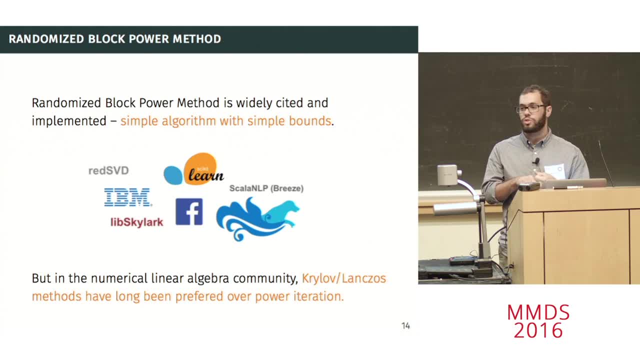 The analysis is simple and the bounds that you get are really simple, so it's easy to use. But the funny thing is is that in the numerical and your algebra community power method is not really the most popular thing. So often power method is replaced sort of by Lanchos and 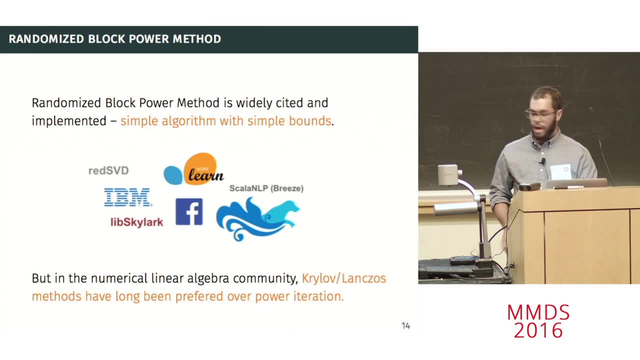 Krylov methods, because they allow you to converge significantly faster. These are sort of polynomial acceleration methods, And so our quest was basically to close the gap between the power method and the power method. And so our quest was basically to close the gap between the power method and the power method. 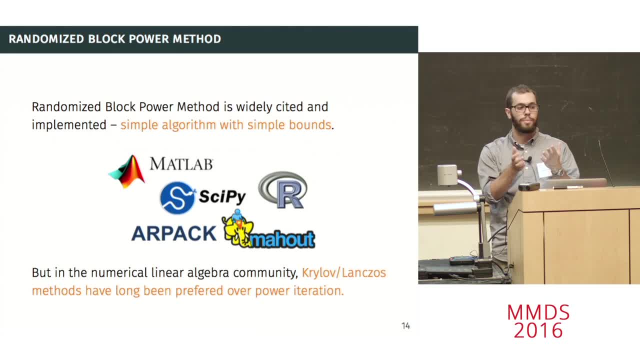 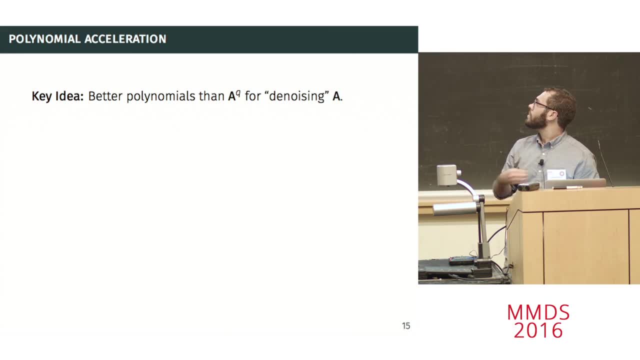 And so our quest was basically to close the gap between the power method and the power method, Like, if this power method analysis has become so popular amongst DNA analysis and machine learning, can we make a Krylov analysis that sort of matches what it does? 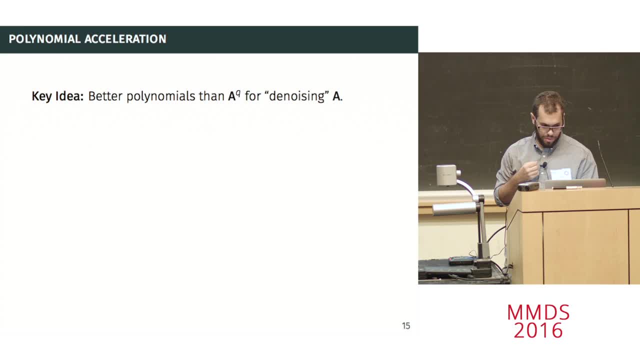 Oh, sorry, I'm going backwards. Ok, And so the basic idea of our view of Krylov methods- and this is sort of the basic idea behind Krylov methods- is that if I'm going to denoise the spectral matrix by raising it to some high power, a 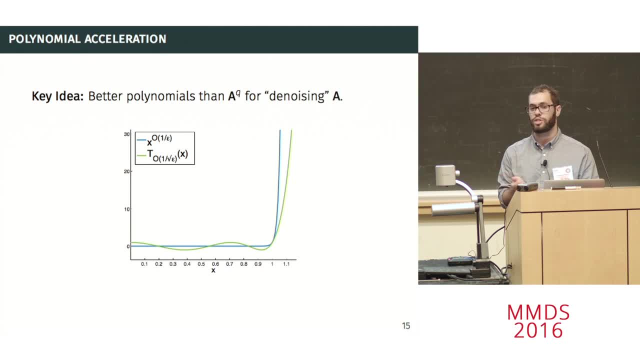 better thing to do instead of raising it to high power. I can actually apply a Chebyshaft polynomial to that Right. Wonderful Thanks, Matt matrix. So if you don't know Chebyshev polynomials, they literally are the 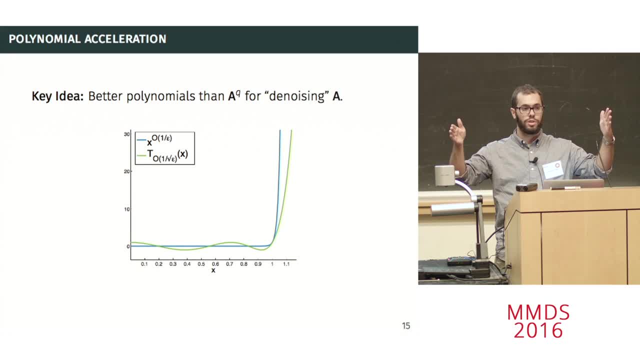 polynomials that are as small as possible in some range, like 1 to 0 to 1, and then as large as possible outside of that range. So they're literally the optimal polynomials for doing denoising in the sense that I'm 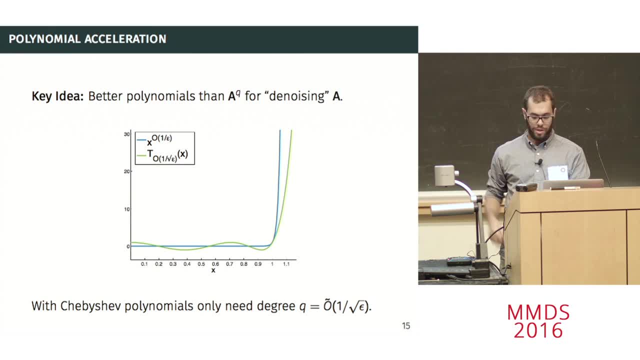 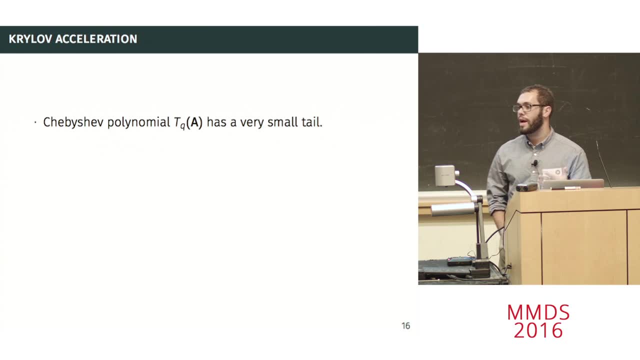 talking about. They depress small values and blow up large values And they can give you like a square root acceleration. So if I needed to set my degree to 1 over epsilon in the power method, I need to set it to 1 over square root of. 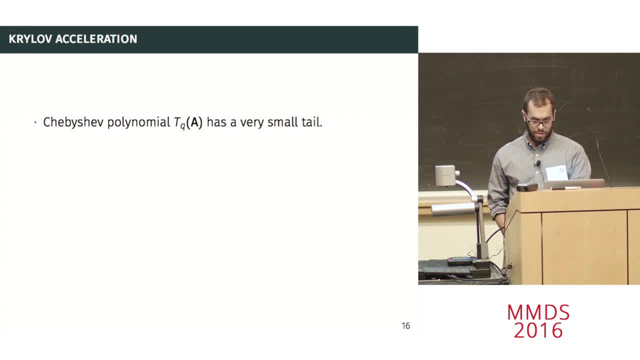 epsilon with a Chebyshev polynomial. So if we can compute a Chebyshev polynomial of our matrix and apply the matrix sketching method to this, we would get a good lower-rank approximation in terms of spectrum there. The issue is that we 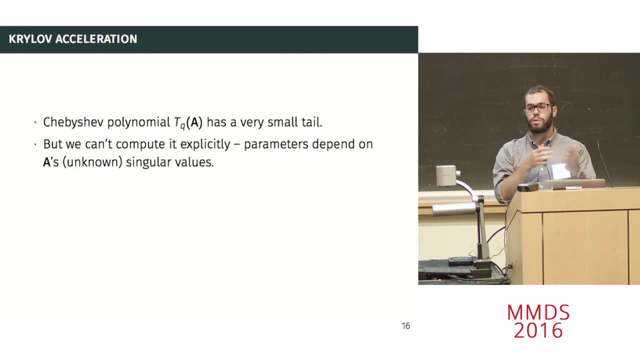 can't like explicitly compute this polynomial. So the actual parameters of the polynomial will depend on the spectrum in our matrix, which we don't know because we haven't done the SVD yet. So we're going to adopt the traditional strategy in numerical methods, which is that we use a Krylov subspace method. 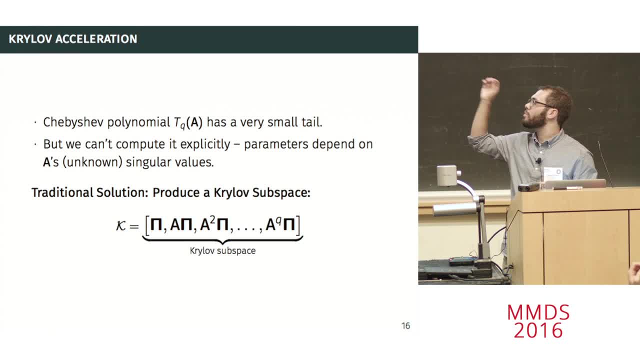 A Krylov subspace is basically, I produce every single polynomial of my matrix applied to like my vectors, my random start vectors, And then I know that my Chebyshev polynomial falls within the span of this Krylov subspace. Every polynomial is just a sum of these. 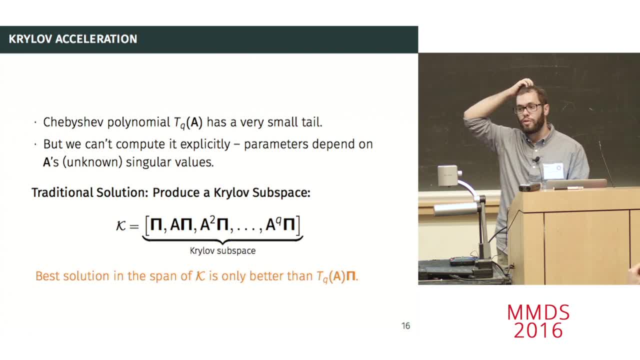 monomials with different weightings. So I know that my Chebyshev polynomial falls in the span of this Krylov subspace. If I can somehow return the best lower-rank approximation within this span, I'm gonna do as well as my. 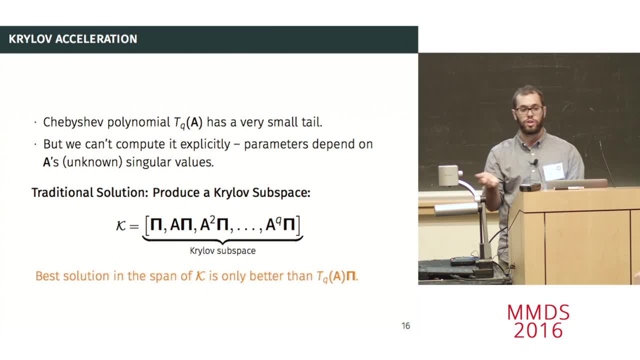 Chebyshev polynomial. I'm never gonna have to have computed the Chebyshev polynomial in the first place and I'm gonna get a good lower-rank approximation. So this is like the trick behind Krylov methods. It's used all over the place in 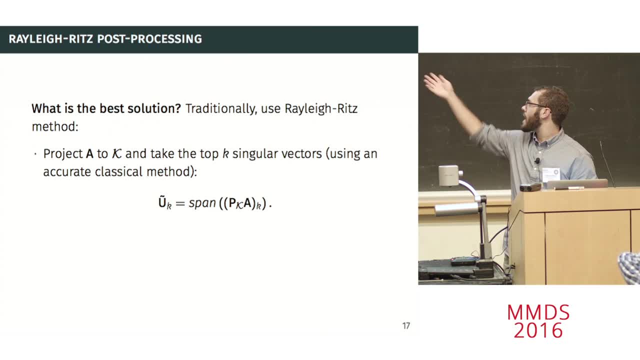 the numerical computation literature. The question is: how do we get this best solution in the span of the Krylov subspace? This was what we really set out to answer. The traditional answer is to use this thing called the Rayleigh-Ritz. 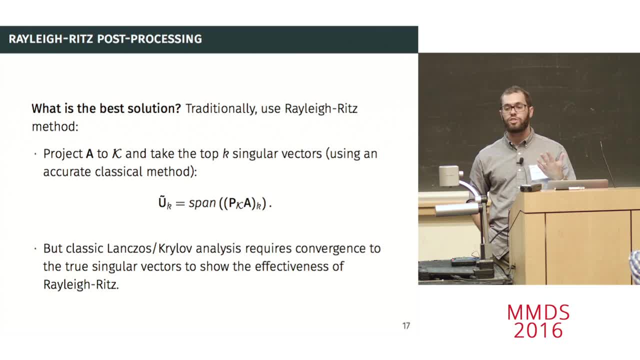 method which I won't go into detail. but basically the idea is you project your matrix to the Krylov subspace and you take the best lower-rank approximation within that projection. Now, unfortunately, like all analysis I've ever seen of the Rayleigh-Ritz method sort of deals with the type of error that 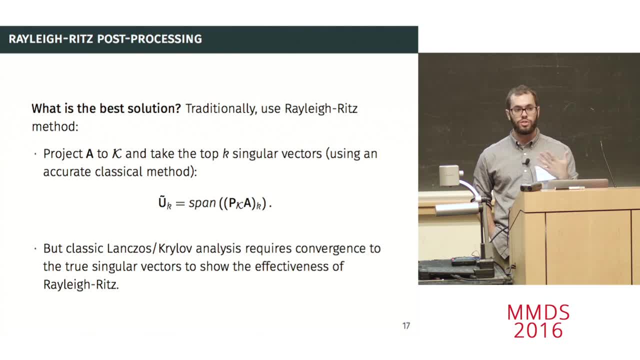 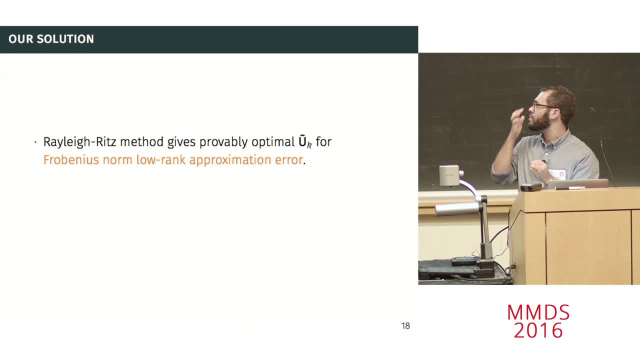 traditional sort of numerical analysis looks at which is the distance between your singular vector and the true singular vectors, And it sort of inherently requires that you have converged to the true singular vectors for these sorts of bounds to go through. So we had to sort of take a different 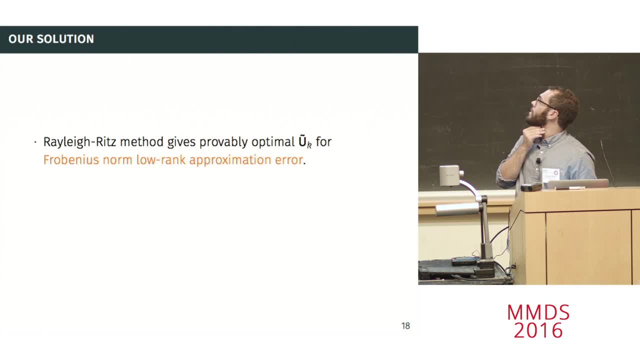 approach and what we basically noticed is that the Rayleigh-Ritz method gives you a provably optimal lower-rank approximation in terms of Frobenius norm for your Krylov subspace. So if I do Rayleigh-Ritz, I'm going to get the best lower-rank approximation in my matrix. 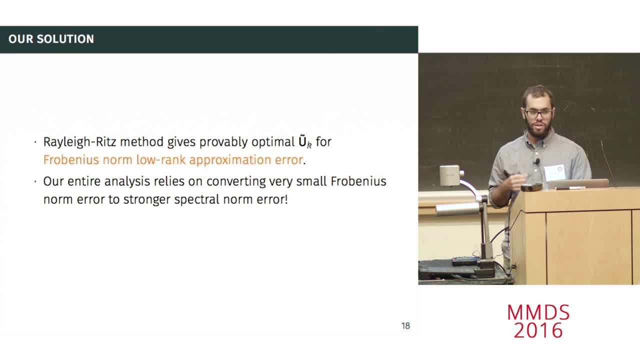 measured in Frobenius norm. that falls within my Krylov subspace. Fortunately, our entire analysis relies on Frobenius norm guarantees. We took these original Frobenius norm guarantees of the sketching methods and we sort of made them stronger by powering up our matrix. So 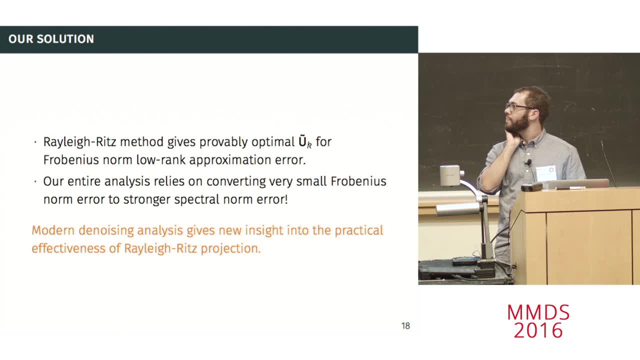 this optimality in terms of Frobenius norm is all we need to get our results And it sort of gives a different analysis of Rayleigh-Ritz. It's like approaching Rayleigh-Ritz from a totally different perspective than traditionally And you're definitely going to be able to. get the best lower-rank approximation in your matrix And you're definitely going to get the best lower-rank approximation in your matrix, And you're definitely going to get the best lower-rank approximation in your matrix And you're definitely going to get the best. 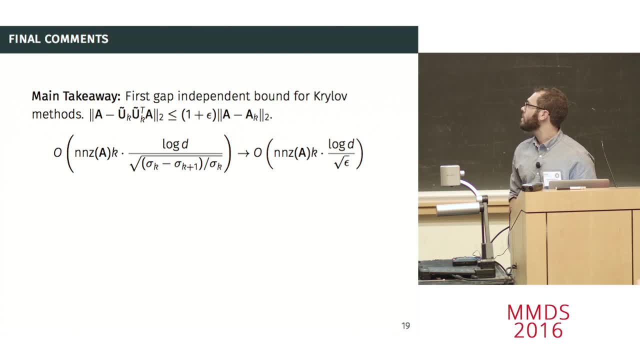 lower-rank approximation in your matrix And you're getting a new result from approaching it from this perspective. So the upshot, really quick, is just that we get the first quote, gap-independent bound for a Krylov subspace method. We basically have number of iterations dependent on epsilon. 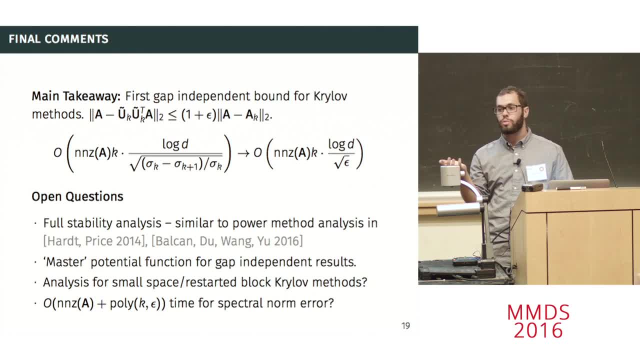 or error parameter, rather than the spectral gap, which can be super small, which you don't have control over, And this accelerates power method by turning an epsilon into a square root of epsilon, which can be significant. There's lots of open questions here, but I'm running low on time so I'm just going to 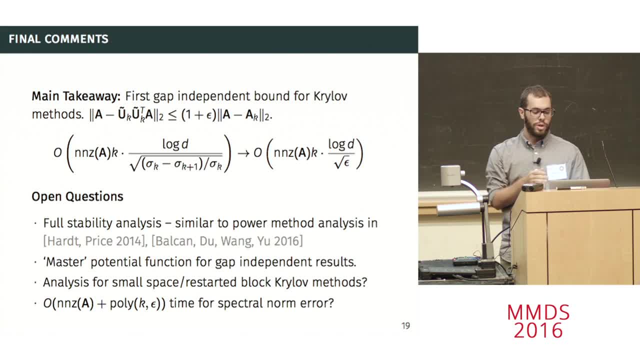 sort of want to survey a couple other ideas. so the upshot of this is all I want to say is that what we basically did was look at what was being done in theoretical computer science and machine learning and combine that what with what had been done in numerical in your algebra, and I think there's tons of ways. 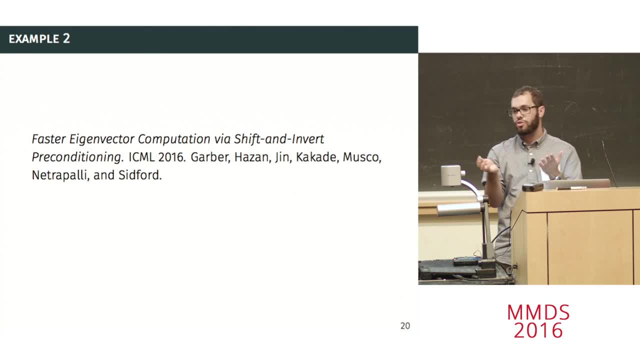 that that can still be done with improving, lowering approximation algorithms and getting stronger theoretical results. let me just give one other example of this real quick. this is a paper at ICML- I guess it was presented yesterday at ICML actually- again on eigenvalue computation via shift and 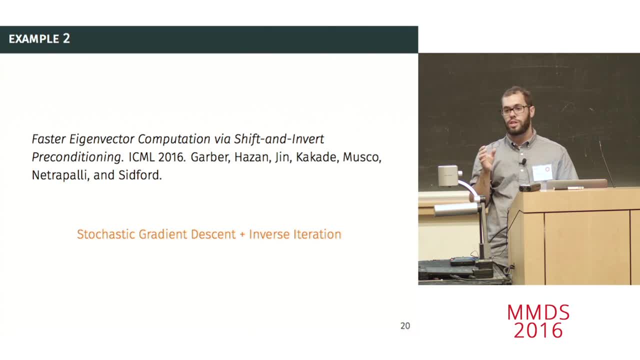 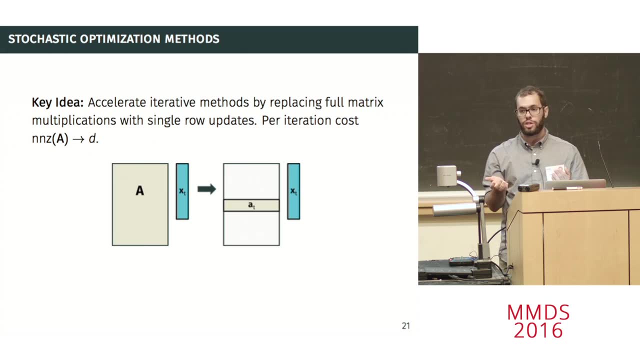 invert preconditioning. the idea here is to basically combine another randomized method, which is stochastic gradient descent, with another classical idea from numerical in your algebra which is like inverse iteration or shifted power method, basically stochastic gradient descent or stochastic methods in general. the way I view them is you're trying to take iterative methods whose base cost 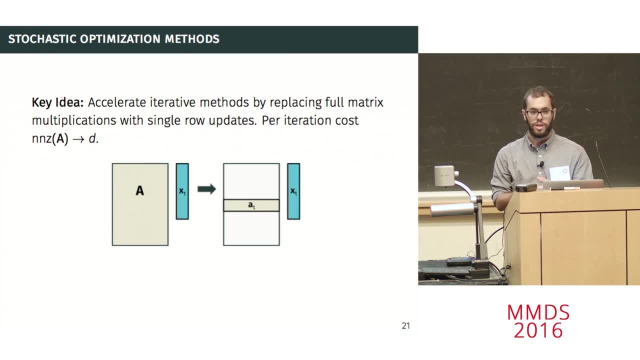 is usually a matrix vector multiply, which costs the number of non-zeros in the matrix, and trying to replace that base cost with a vector vector multiply, you sample one row of your matrix and you a vector vector multiply. by accelerating the number of iterations you can get all. 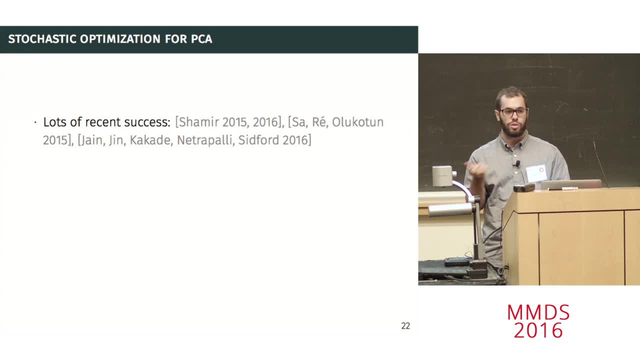 sorts of speed ups, you can get better results in streaming settings, distributed settings etc. so these things work really well in practice. there's lots of interesting theory and so obviously there's an interest in using them for doing principal component analysis. there's lots of papers on this. 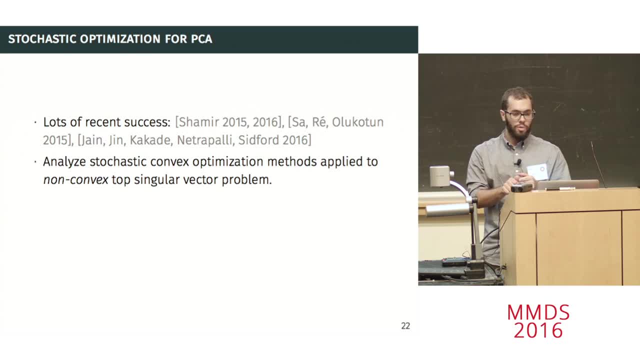 and sort of the traditional viewpoint is that what you can do is computing the top eigenvector of a matrix or the top singular vector is a non-convex problem, but the hope is that it's simple enough that you can sort of analyze it and show. 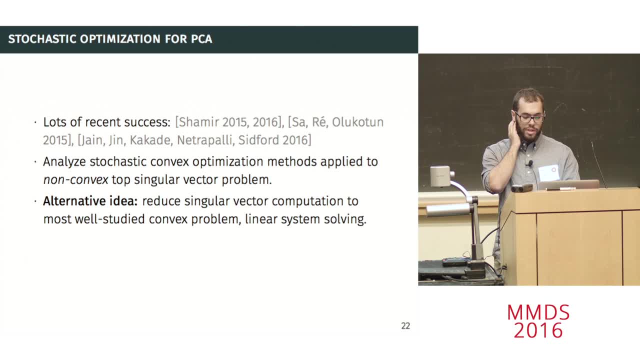 that these convex optimization techniques still work well. what we did was, instead of trying to analyze this non-convex problem, we just said: let's reduce this problem to the most popular convex problem, which is basically linear system solving. so I want to reduce getting the top eigenvector of matrix to 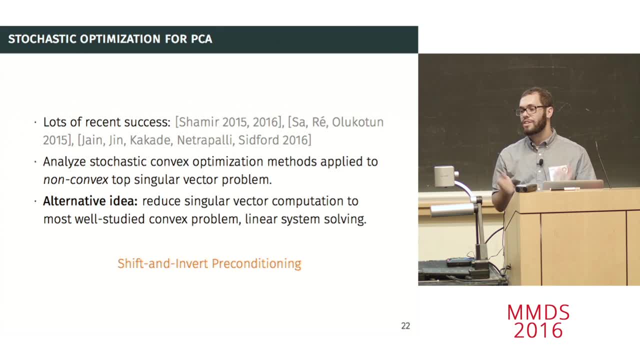 solving a linear system in that matrix and this is like a classic idea in numerical linear algebra called shift and invert preconditioning. basically, you choose a specific matrix such that when you compute the inverse of that matrix, if you apply power method, it's gonna give you very fast convergence top eigenvector. I'm gonna skip all the. 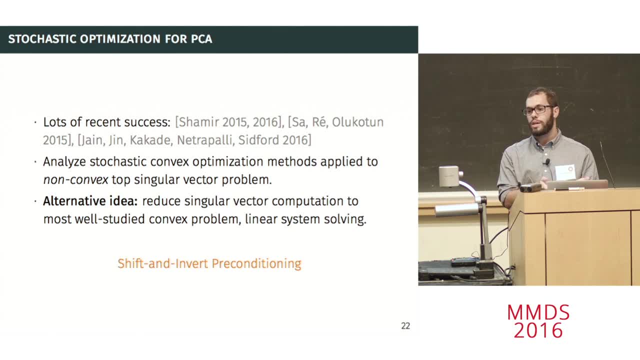 details of this, but the idea is basically that we then do our invert method, the step of shift, and invert preconditioning using stochastic gradient methods, basically black box- and then we're able to show speedups for computing the top eigenvector that get all sorts of trade-offs with the size of 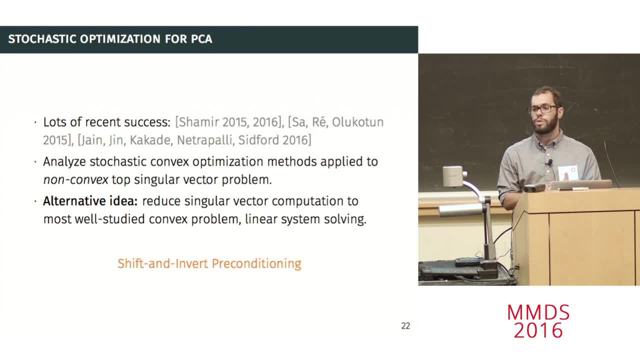 your matrix or spectrographs etc. and I think we sort of contribute two things other than just combining the two ideas- is that we're sort of analyzing these stochastic gradient methods specifically for use in the shift and inverted setting. Two is that these sort of methods give much looser guarantees than traditional linear system. 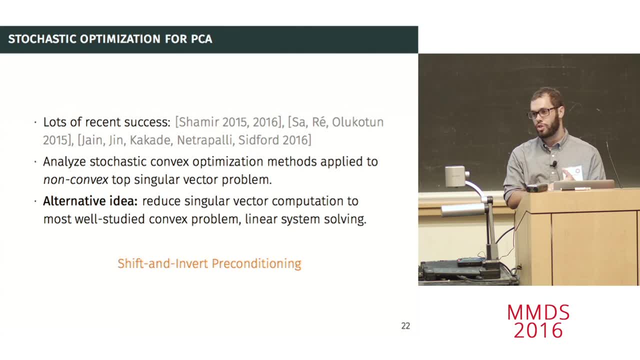 solvers, and so we have to sort of redo the analysis of shift and invert preconditioning and make it significantly more robust than you would find in a traditional analysis. So in doing this we sort of open up this method to being used for a much broader range of solvers. 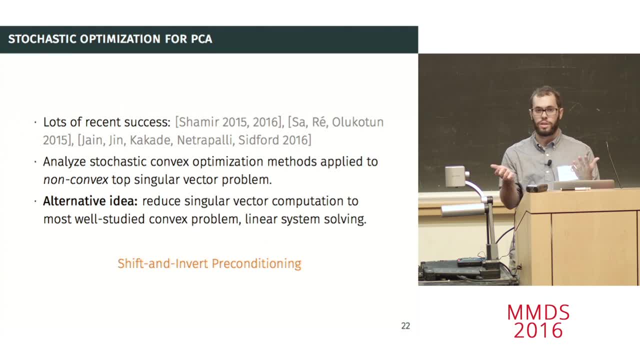 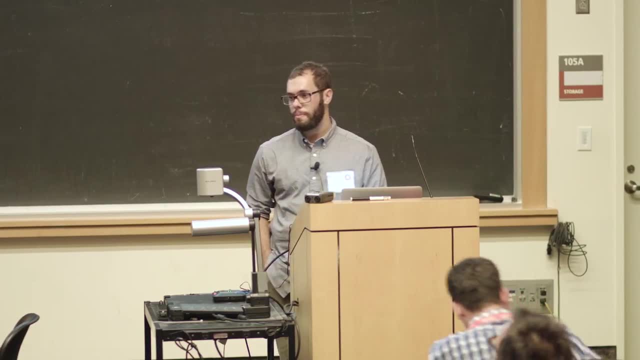 than what would typically be considered by people in numerical linear algebra. So that's basically. I think I'm going to cut it off there. Yeah, that's it.